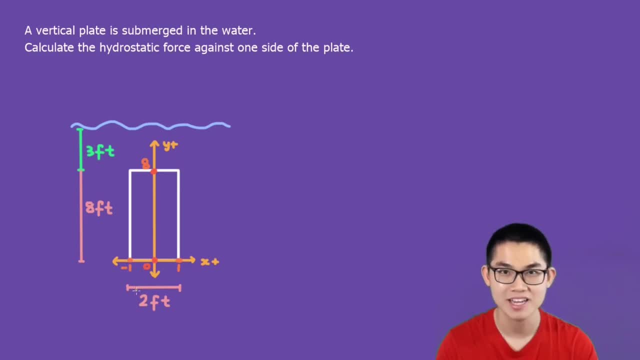 the distance from here to here is also one, so that's why this is negative one here. The idea behind calculating the hydrostatic force is that you calculate the force that this stripe of water is acting on the object and then you calculate the force that this stripe is acting on the object. 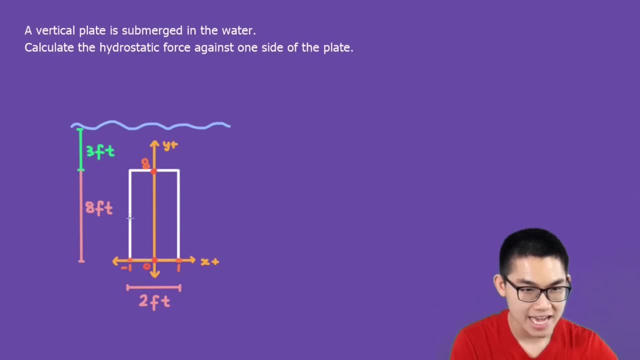 and then the force from this one, then this one. So you get the idea we keep doing that until we reach the top, like this, and then we add all of those forces together and that will give us the hydrostatic force. Here I draw this line to represent our 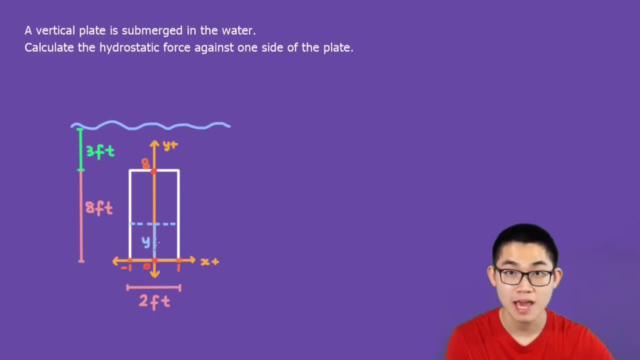 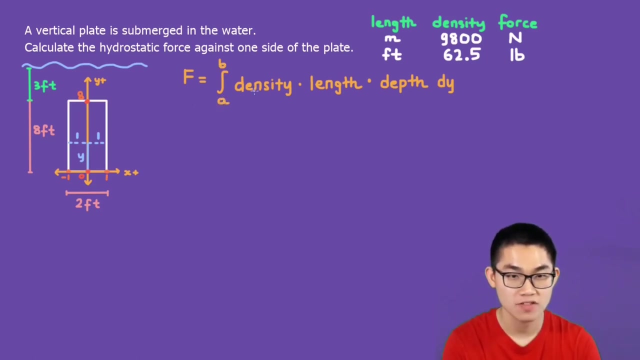 stripe and the distance from the center to this stripe is y. Now we also know that from here to here is one, and from here to here the distance is also one. This is the formula to calculate the hydrostatic force and, as you can see, we have the integral from a to b of the density. 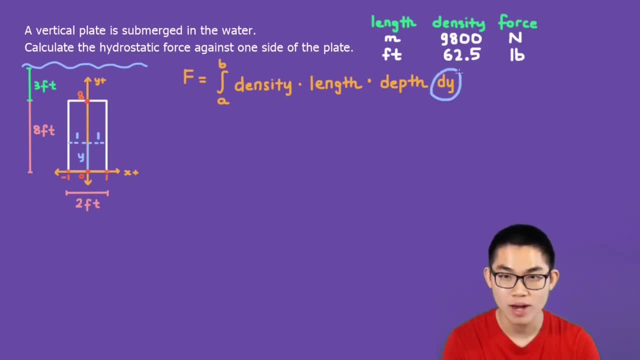 times the length, times the depth and dy. So we want this function to be in terms of y, and I'm going to show you how to find these parameters. So, first of all, if the length is in meters, then the density will be 9800, it's just a number that you have to know. 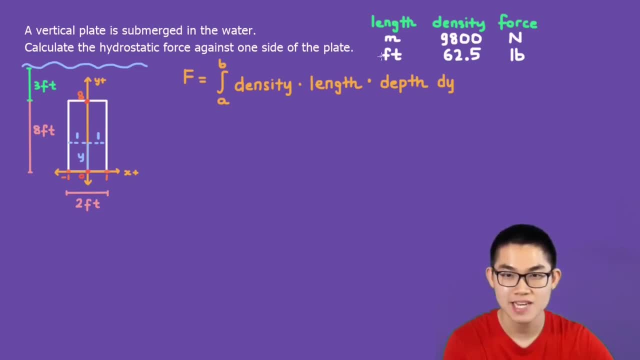 and the force will be in newtons, Whereas if the length is in feet, then the density will be 62.5, and the force will be in pounds. But what is from a to b? Well, a is zero and we want to calculate the force up until the very top, which is eight. 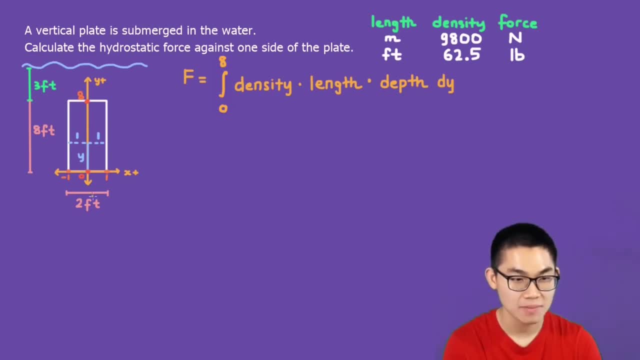 What is the density? Well, as you can see, this problem is in feet, so the density will be 62.5.. What is the length? Well, the length is the length of the stripe from here to here and, as mentioned before, it's going to be two, because this stripe has the same length as the 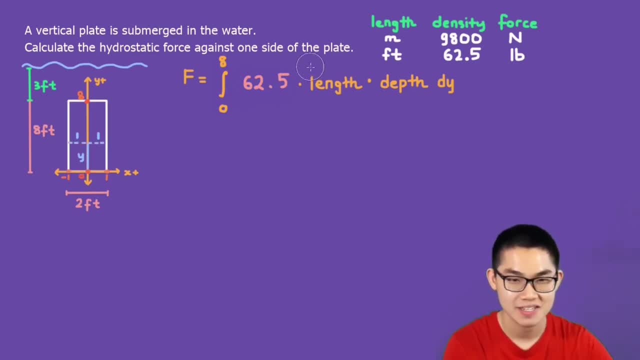 width, and therefore it's just two. Last but not least, what is the depth? Well, what does depth mean? The depth means the distance from our stripe to the surface of the water. Now we want to calculate this distance. so what is this distance? First of all, we know that the 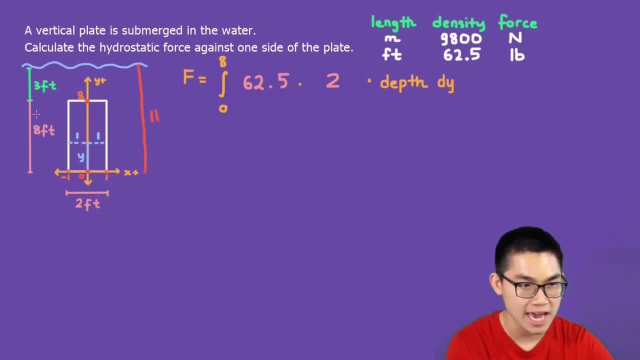 distance from here to here is going to be 11, because we have 8 plus 3, that's going to be 11.. The goal is to calculate this distance, so that's going to be 11 minus this distance, which is y. 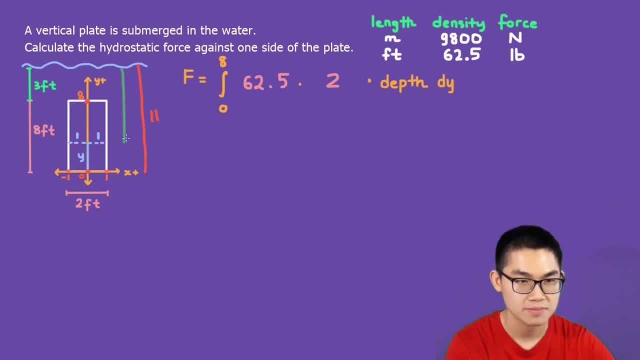 11 minus y. that's going to give you this. This integral is very easy to solve, so let me save you your time and just say that this is equal to the distance from here to here, and that's going to give you this. 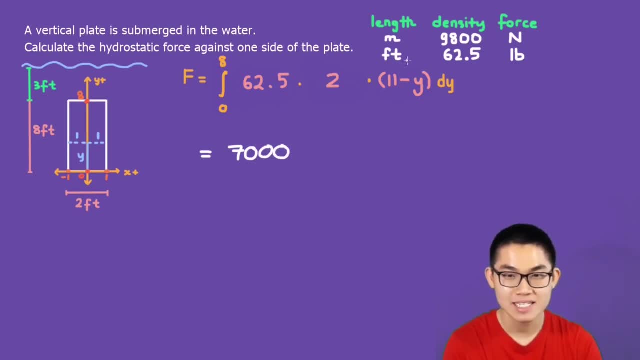 And what is the unit? Well, this problem is in feet, so the unit or the force is in pounds, so let's say pounds, and that is the answer to this question. In the next video, I will show you how to do the problem where the shape is a triangle. 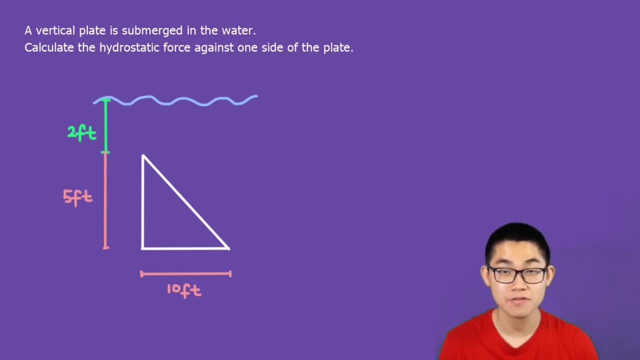 In this video I'm going to show you how to calculate the hydrostatic force acting on an object submerged in the water. So, for example, here we have an object or a vertical plate that is submerged in the water. It takes form as a triangle and we know that the height 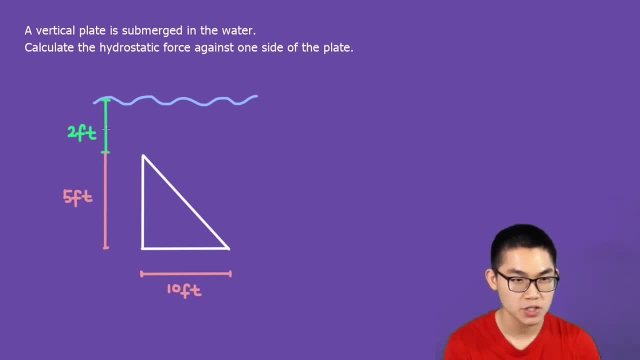 is 5 feet, the width is 10 feet and it's submerged 2 feet into the water. The first thing I'm going to do is put the x and the y-axis onto this triangle. So, as you can see, I put the x-axis on the base of the triangle and the positive direction is to the right. 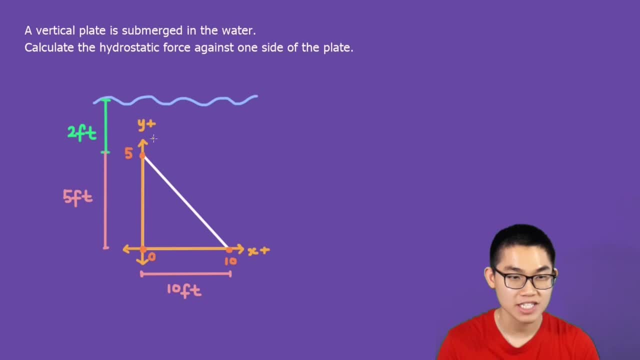 For the y-axis. I put it on the side and the positive direction is upwards. Also, because the width is 10 feet, the horizontal axis is on the right and the horizontal axis is on the left, So this point is zero at the center and then this point is going to be 10,. 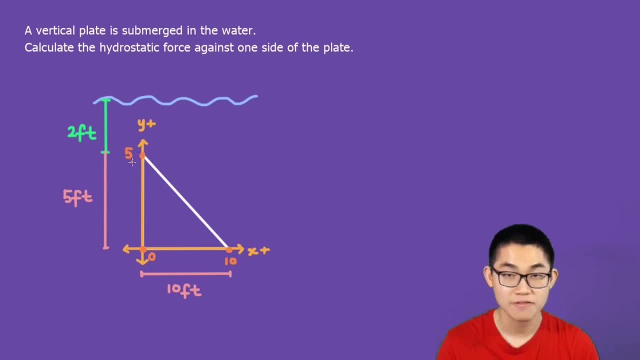 and since the height is 5, we know that this is going to be 5 here. To calculate the hydrostatic force, we have to calculate the force of this stripe acting on the triangle, and then we have to calculate the force of this stripe acting on a triangle. 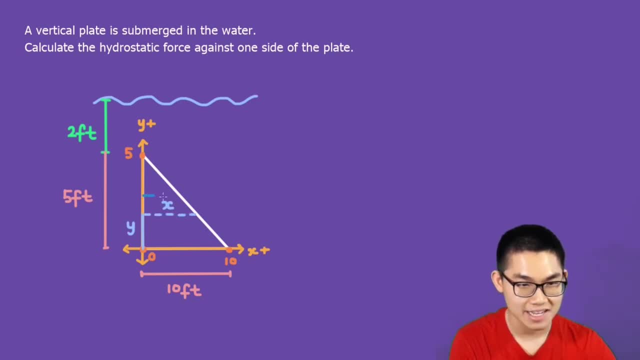 and then this one, and then this one, and you get the idea We're going to calculate until we reach the very top, and then we're going to add all of those forces together, which gives us the hydrostatic force. So I'm going to draw this as our stripe. It's going to represent 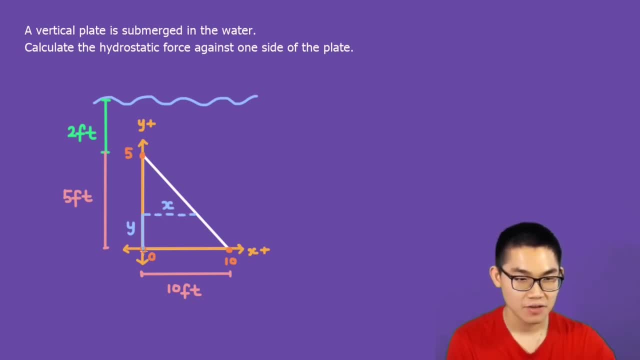 the stripe that we're currently at and the height from the center to this stripe. we're going to call it y. So what is this length? What is the length of this line? Well, we don't know what it is, so we're just going to call it x. And here is the formula to calculate the hydrostatic force. 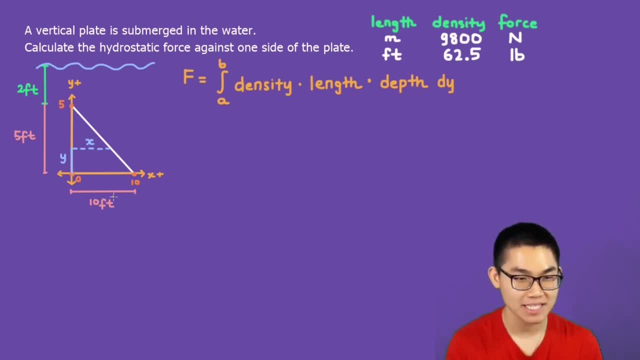 as I've shown you in the previous video, and since the problem is in feet, the density will be 62.5, and the answer or the force will be in pounds. So what is a and b? Well, a will be the base of. 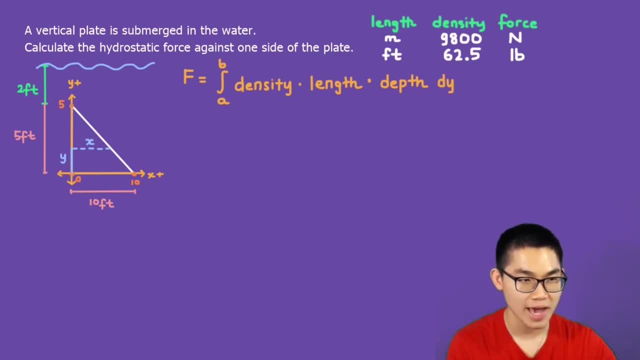 the triangle which is here at zero and b is the top. So a is zero and b is five. How about the density? Well, the density will be 62.5, because the problem is in feet. What is the length? Well, it's very easy. So the length is the length of our stripe, like that, and as you can see. 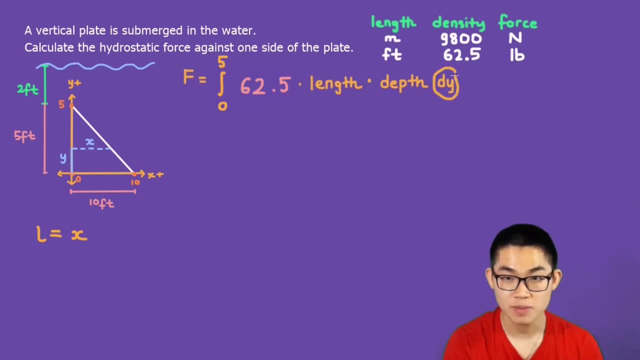 it's equal to x, but our formula wants everything to be in terms of y, So let me show you how to convert the x into a y From this diagram. we know that this point is zero five. right, It's zero five. 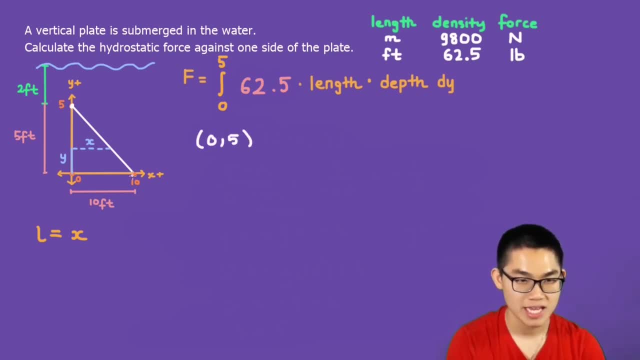 so we write it out. So we have zero five and this point is ten zero. Let's calculate the slope. We have five minus zero over zero minus ten. That gives us five over negative ten, which is equal to negative one over two. So we have five minus zero over zero minus ten. That gives us five over negative ten, which is equal to negative one over two. 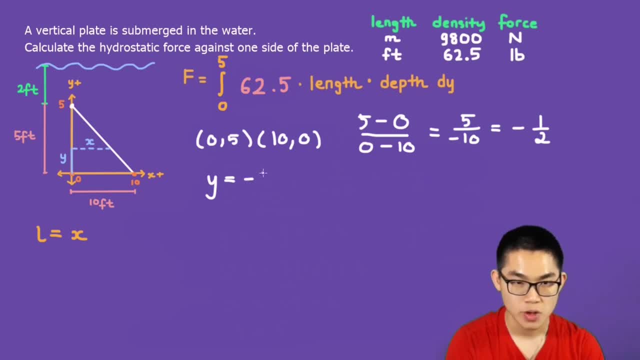 Using the slope formula, we have: y is equal to negative one over two x plus b, and we're going to substitute in one over these two points. So let's substitute in this one: y is five, x is zero, so negative one over two times zero plus b, and therefore we have: b is equal to five. 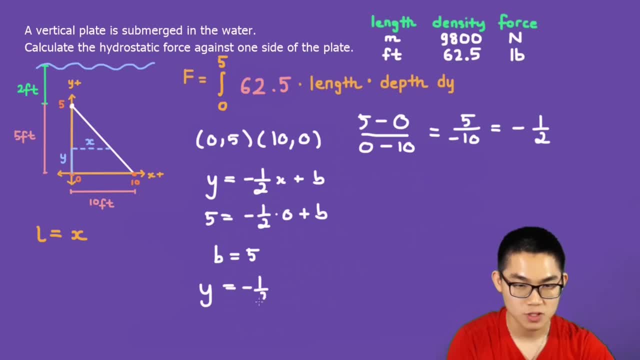 And the equation is: y is equal to negative one over two x plus five. Let's solve for x, We have: y minus five is equal to negative one over two x. We multiply both sides by negative one, We get negative. y plus five is equal to one over two x. Multiply both sides by two: We get negative. 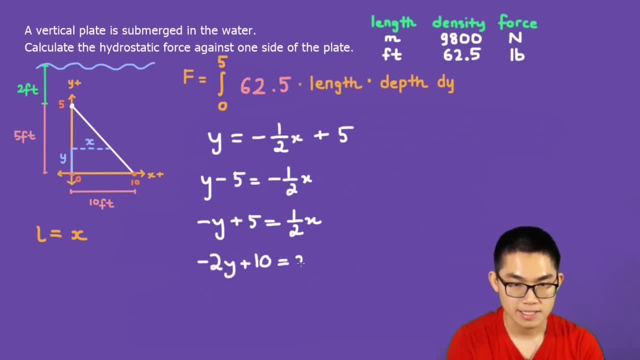 two y plus ten is equal to x, And so l over the length is just ten minus two y. We are almost done. How about the depth? Well, the depth is the distance from our stripe to the surface level of the water. so this distance, here We know that let's use y. 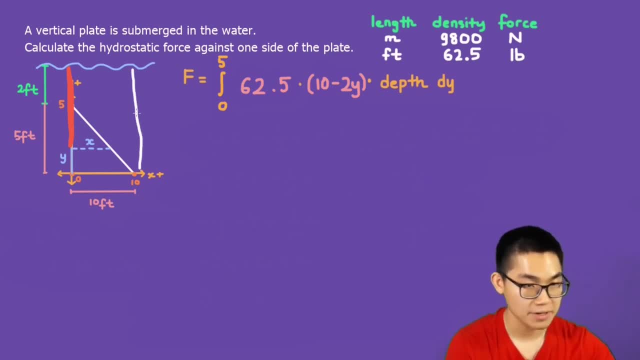 we know that this distance from here to here is going to be seven. It's going to be seven because we have five plus two. That's going to give us seven. So if we take seven and we subtract this distance, which is y, then we get the orange stripe, which is seven minus y. 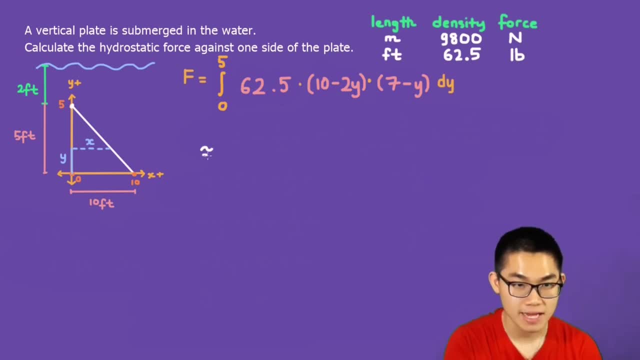 This integral is very easy to solve, so let me save time And give you the answer. So after you do it, you should get 8333.33.. And what is the unit? Well, the problem is in feet, so the force or the unit will be in pounds. 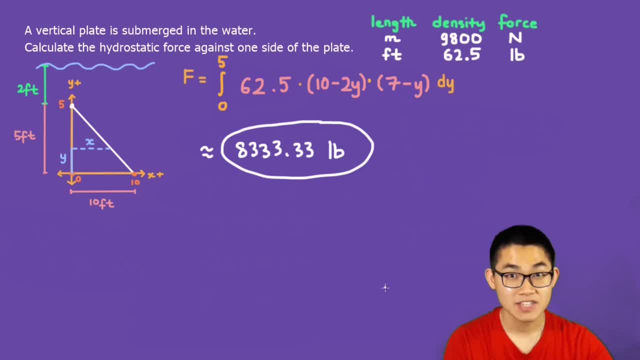 And that is the answer to this question. In the next video, I will show you how to calculate the hydrostatic force when the shape is a trapezoid like this. In this video, I'm going to show you how to calculate the shape of a trapezoid. 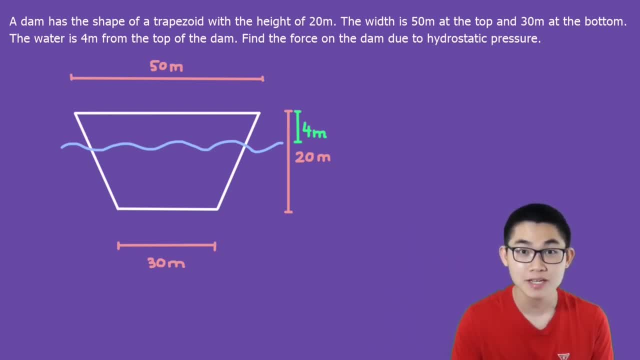 I'm going to show you how to find the hydrostatic force on an object submerged in the water. So the problem is: a dam has the shape of a trapezoid with the height of 20 meters. The width is 50 meters at the top and 30 meters at the bottom. 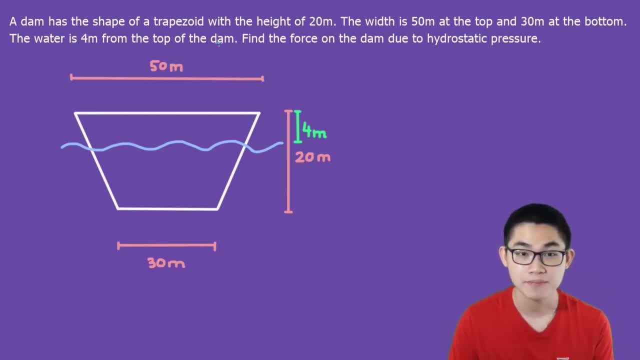 The water is four meters from the top of the dam. We have to find the force on the dam due to hydrostatic pressure. So I've drawn this diagram and our trapezoid is submerged in the water, but not all the way. 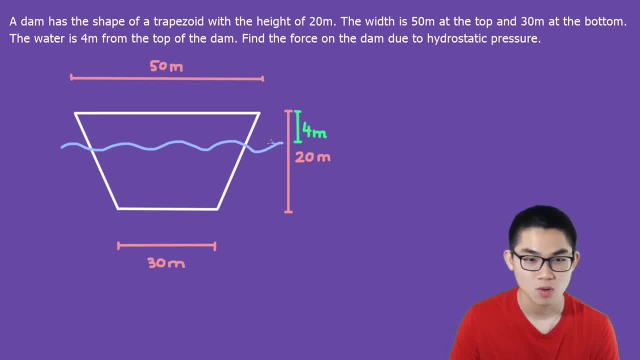 there's four meters between the top and the surface of the water. The height is 20 meters, as you can see, and the width is 50 meters at the top and 30 meters at the bottom. The first step is to put the x and the y-axis on this shape. 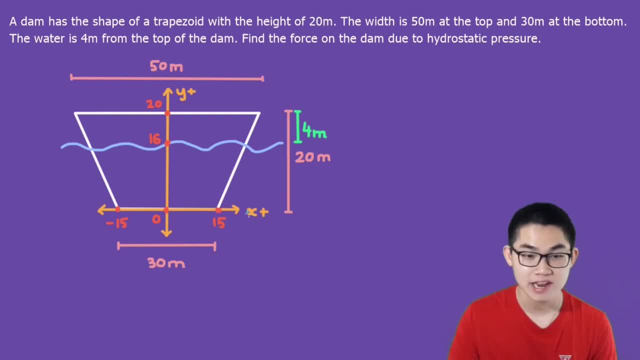 So I've put the x-axis at the bottom of the trapezoid and here is the positive direction. The y-axis is in the middle of the object and the positive direction is upwards. And because the distance here is 30 meters, then we know for sure that the distance from here is 15,. 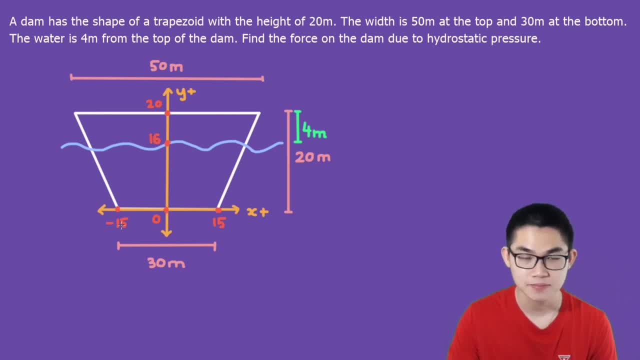 here and over here is also 15, so this is negative 15.. The height is 20 meters, so you can see this is 0, this is 20, and because there's a distance of 4 meters from here, then we know that this value is 16.. 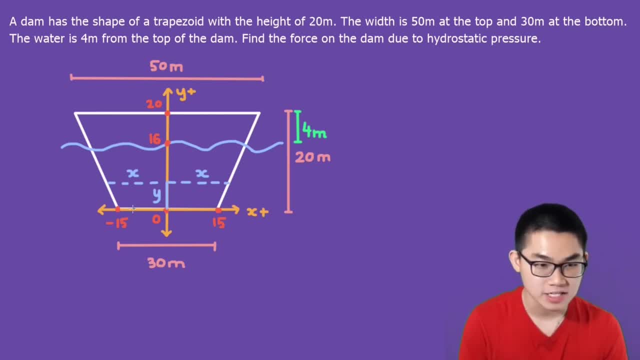 To calculate the hydrostatic force. the idea is to find the force of this stripe acting on the object and then find the force of this stripe acting on the object, and then the force of this stripe, then this stripe. So you get the idea. we keep doing that until we reach the surface of the 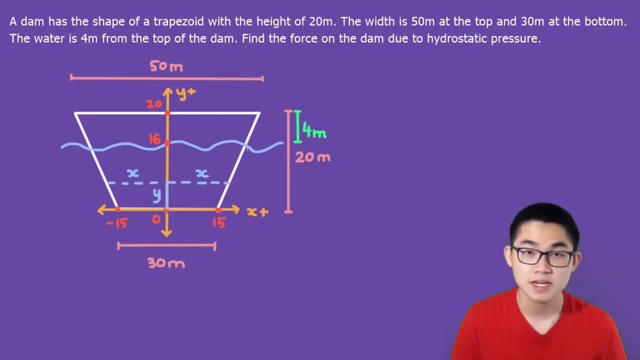 water, and then we add all of those forces together, which gives us our hydrostatic force. So let's say that this is our stripe. let's say this is our stripe, then the distance from the center to our stripe is y, the distance from here to here is going to be x. but we also know that 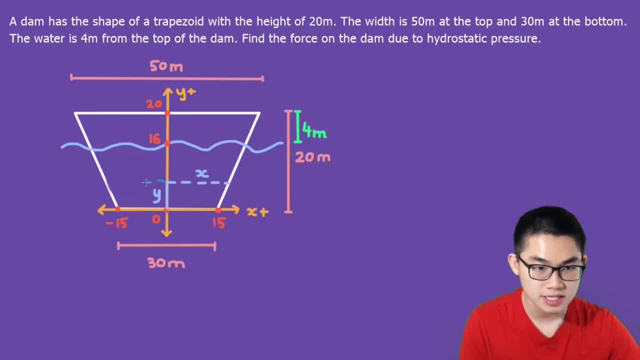 because the y-axis divides this shape in half. then the distance over here is also x, so the total distance of the stripe, or the length, is equal to 2 times x. And here is the formula to calculate the hydrostatic force. and let's solve this formula. 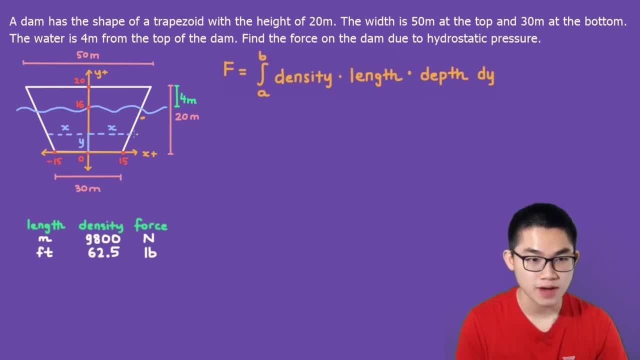 together. So what is a and what is b? Well, we want to find the hydrostatic force act because of the water, which is from here to 16, right, So a is 0 and b is 16.. What is the density? Well, I've put. 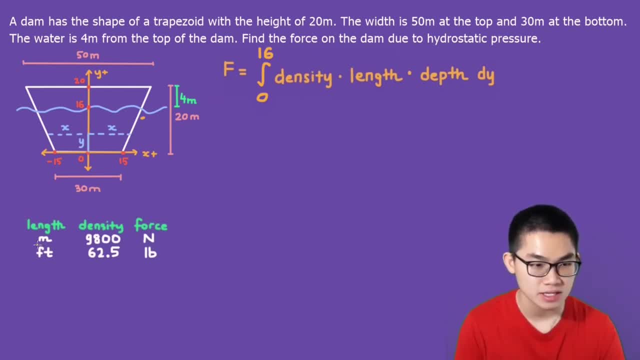 this table here, and because the problem is in meters, then the density will be 9800.. How about the length? Well, we want to find the length of the stripe and, as mentioned before, it's going to be 2x, But the formula wants everything to be in terms of y. 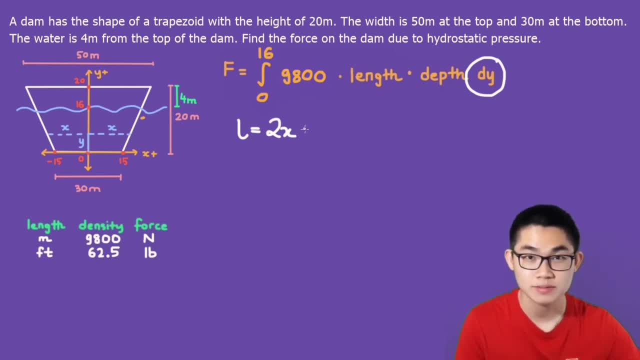 so we have to convert the x to the y, and let me show you how to do it. If you look here, this point is going to be 15, 0, right? This is the point on the x and the y-axis. 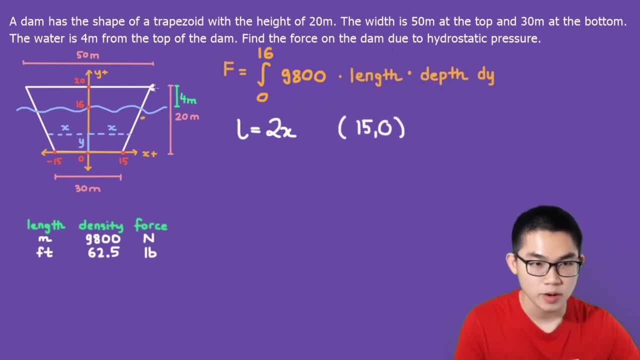 so let's write it out. How about this point here? Well, the distance from here to here is half of 50. We know that from here to here is 50,, so from here to here is 25, and the height is 20.. 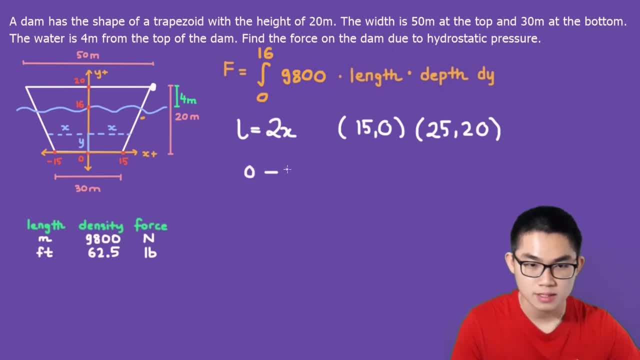 Let's calculate the slope. We get 0 minus 20 over 15 minus 25.. That's going to give us negative 20 over negative 10, which is going to be 2.. And using the linear formula, we have the slope 2x. 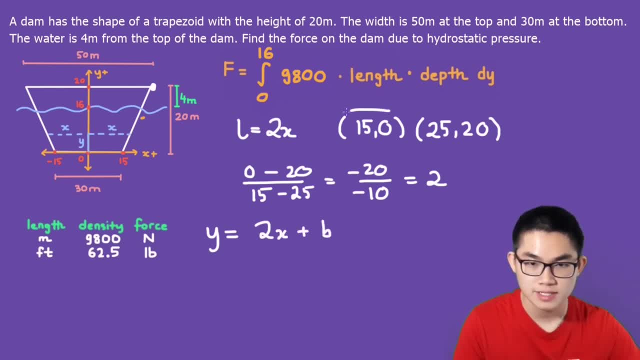 plus b and we have to substitute one or these two points. Let's substitute this one, so the y is 0, x is 15, so 2 times 15 plus b, b is going to be negative 30, so we get: y is equal to 2x minus 30. 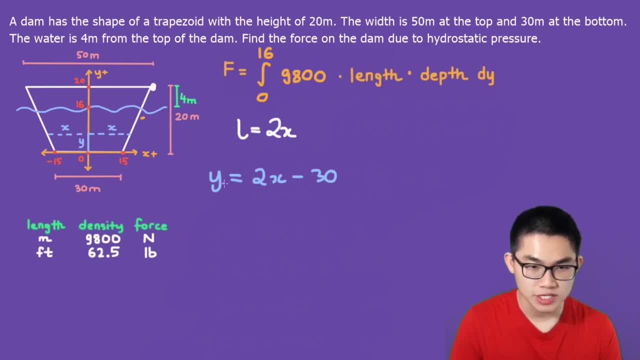 Let's solve for x. So in this equation that we just found out, we get: y plus 30 is equal to 2x, and then x is going to be 1 over 2y plus 15, so the length is 2x, which means 2 times. 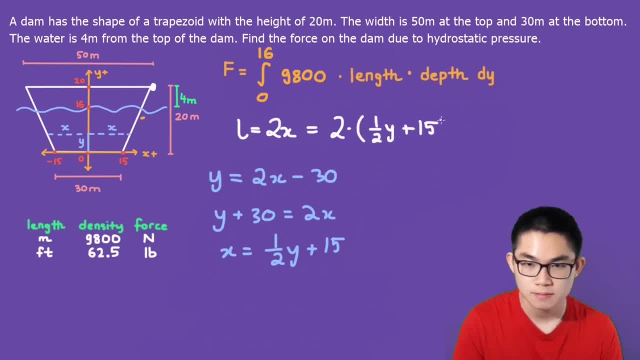 1 over 2y plus 15.. That's going to be y plus 30.. Let's put it back into the length here. Last but not least, we need to find the depth. So the depth is the distance between our stripe. 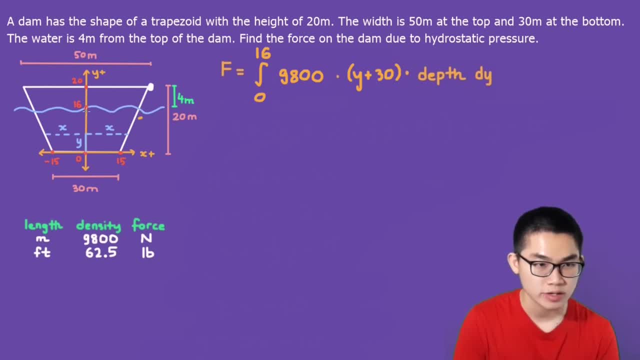 to the surface level of the water. So that's going to be this distance. We want to find this depth right there. Well, first things first, we know that the distance- let's use yellow this time- so the distance between the x-axis to the surface level of the water, that's going to be 16,. 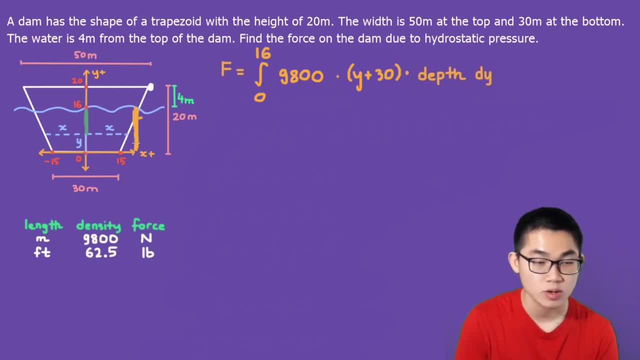 right, You can see here, that's 0,, that's 16, so the yellow distance is going to be 16.. Well, if we take the yellow distance and we minus y, we're going to get the green distance. So the depth is just basically 16 minus y. This integral is very easy to do, so let me 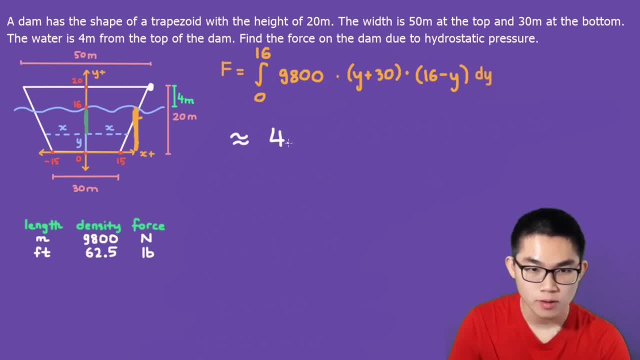 save you your time. and after you solve it, you should get 4.4 times 10 to the power of 7.. And And what's the unit? Well, looking at this table, the problem is in meters. so the final answer is the force, which is newtons. 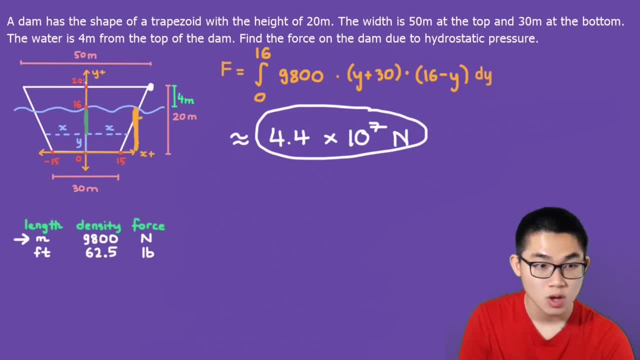 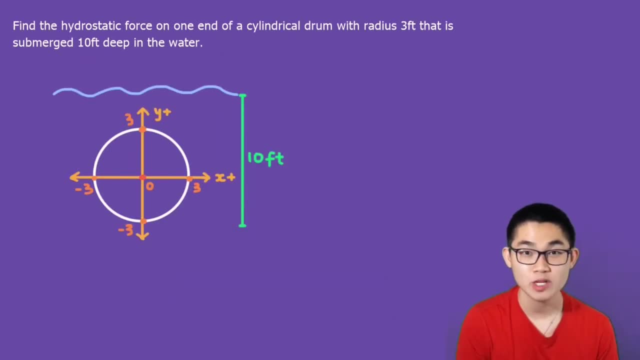 In the next video I will show you how to calculate the hydrostatic force when the shape is a circle. In this video I'm going to show you how to calculate the hydrostatic force acting on a circular object submerged in the water. So the problem says: find the hydrostatic force on one end of the cylindrical drum, which is basically just a circle with radius 3 feet that is submerged 10 feet deep in the water. 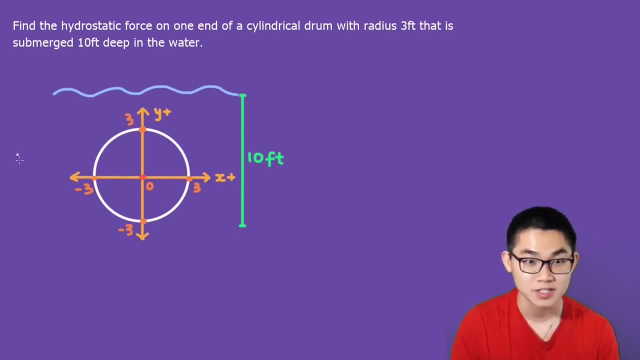 So you can see here, the distance from here to here is 10 feet, as shown in the textbook, and the radius is going to be 3.. The first step is to put the x and the y axis onto this diagram, and the way to do it is you put it at the center of the circle. 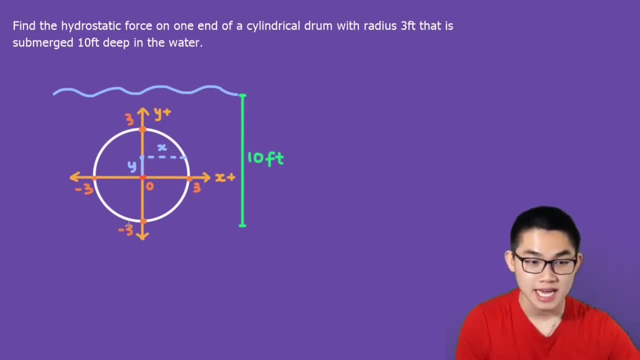 So the idea behind this is to put the x and the y axis onto this diagram, and the way to do it is you put it at the center of the circle. The idea behind finding the hydrostatic force is that you find the force of, let's say, this stripe acting on the circle. 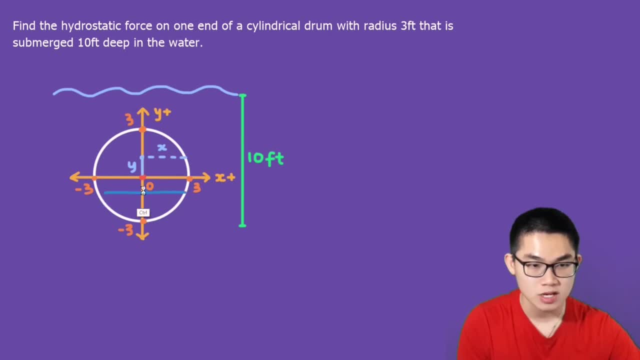 then the force coming from this one, then this one, then you keep doing it until you reach the very top of the circle. Then you add all of those forces together, which gives us the hydrostatic force. Let's say that we're currently at this stripe. 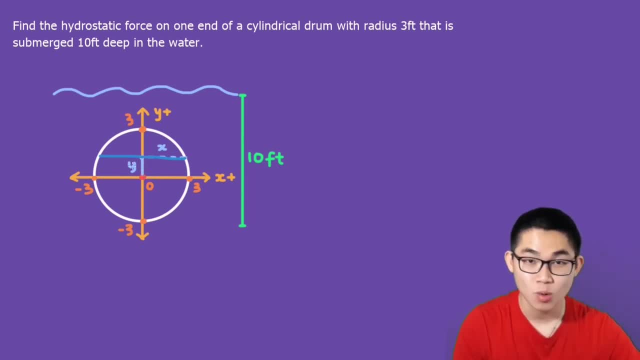 Then the distance from the center to the stripe is y, that's the vertical distance, and the distance from here to here is going to be x. But since the y axis divides the circle in half, we also know that the distance over here is also x. 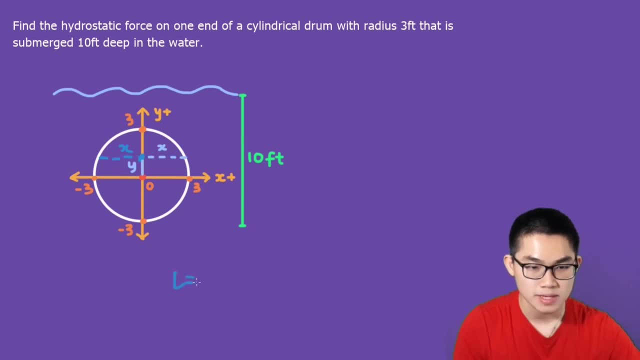 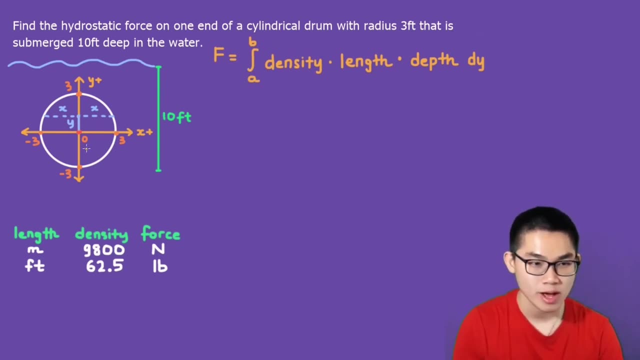 So the total length of the stripe is going to be 2x, And here is the formula. Now let's find a and b first. Well, we want to find the hydrostatic force acting on the object from here up until the very top of the circle. 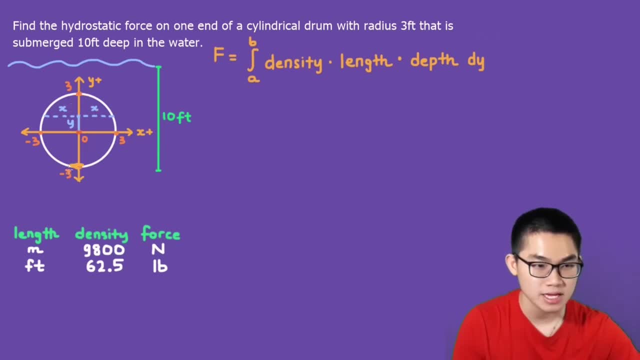 So that distance is going to be from negative 3 to positive 3.. So a is negative 3 and b is positive 3. Since the problem is in feet, then the density will be 62.5.. The length of the stripe from here to here is going to be 2 times x. 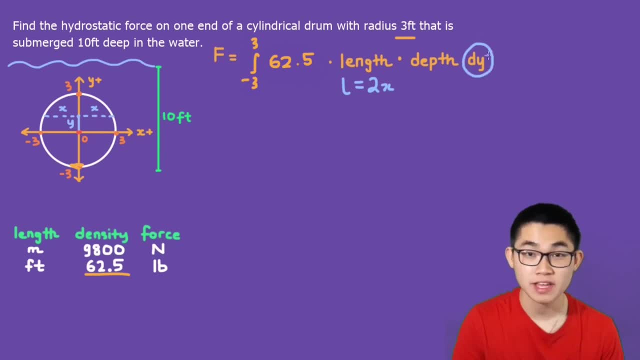 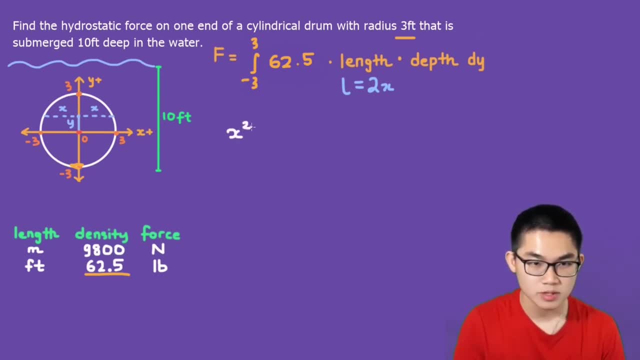 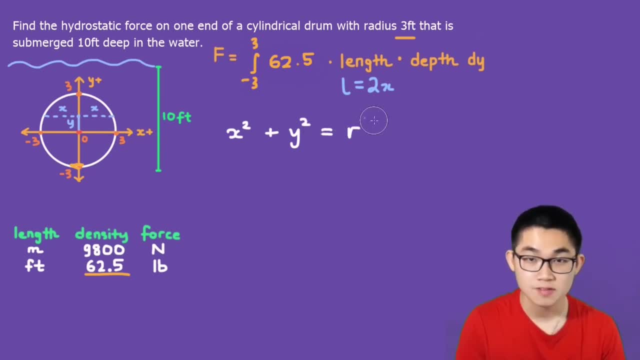 And since the radius is 3, then 3 squared gives us 9.. We simply solve for x, So we get: x squared is equal to 9 minus y squared. We take the square root on both sides and that's going to give us the square root of 9 minus y squared. 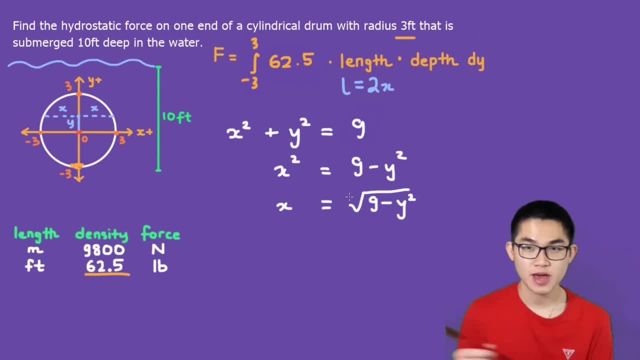 Here we only take the positive, because if you imagine you have a ruler, only makes sense to say that the length of the ruler is positive and not negative. we found x, so the length will be 2 times the square root of 9 minus y square. let's put it back into here. 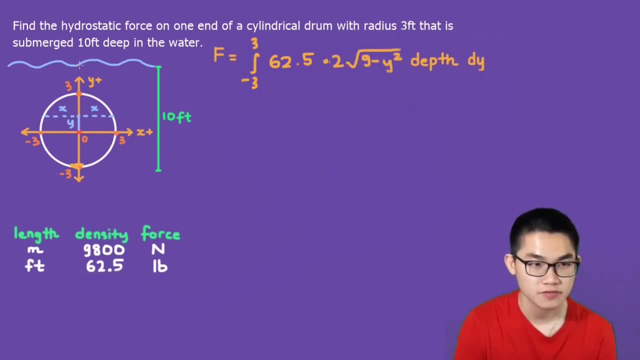 the depth is the distance from our stripe to the surface of the water. so it's going to be the red distance here. we know that. from here to here, what is this distance? it's 10 minus 3. that's going to give us 7, because the radius is 3, right, and we know that this is 10. so 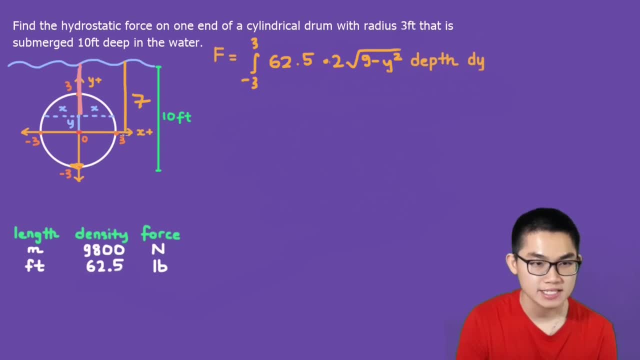 this one has to be 7.. now if you take this length and you minus this length, it's going to give us the red length. so the red length, or the depth, is just 7 minus y. let's solve this integral together. so we take this, multiply by 2 and then we take it outside of the integral because it's a constant. 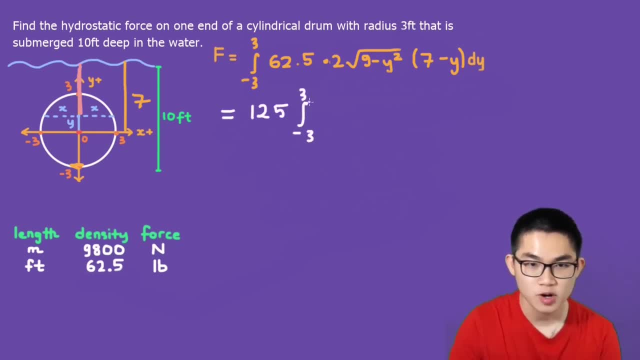 so you get 125 times the integral from negative 3 to 3 of the square root of 9 minus y, squared times 7 minus y dy. we need to solve this. we need to simplify this. we take this multiply by 7, then we take this multiply by negative y. that's going to give us: 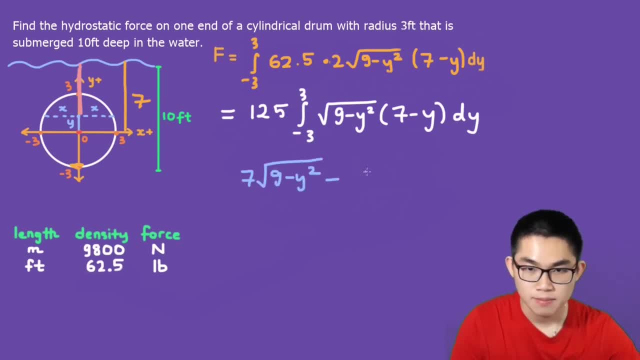 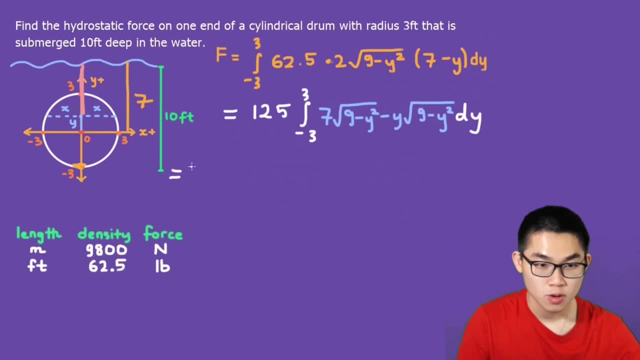 7 times the square root of y minus y square minus y times the square root of 9 minus y squared. this is equal to 125 times the integral from negative 3 to 3 of 7 times 9 minus y squared times 9 minus y squared dy minus the integral from. 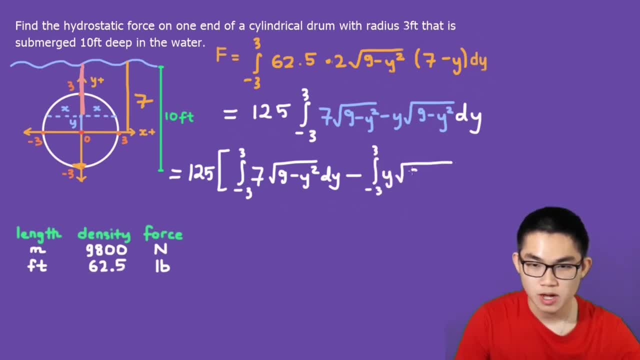 negative 3 to 3 of y times the square root of 9 minus y squared. and why am i doing this? because you can solve each one as a sub problem and then we can combine them together. it's way simpler this way. in order to solve this problem, you need to know this theorem, which is the integral of symmetric. 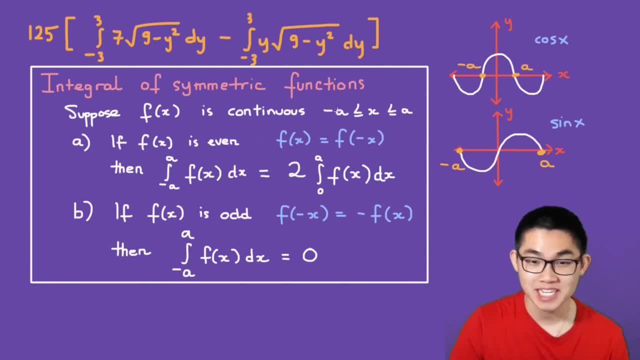 functions. if f is a continuous function from negative a to a on the x-axis, then if f is even, which is just this formula, if you can show that this formula is true, then the integral from negative a to a of f of x dx is equal to 2 times the integral of 0 to a f of x dx. so what exactly? 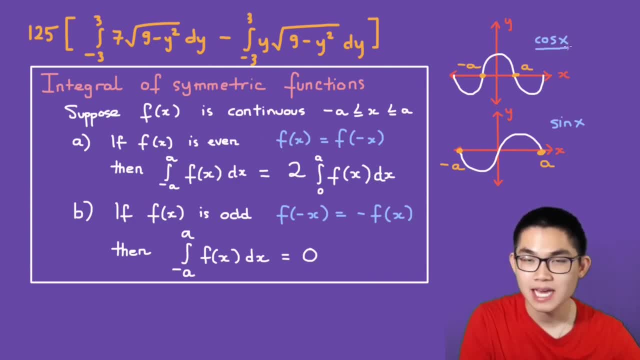 does this mean? for example, cosine is an even function, because if you look here, from negative a to a, the area on this side is equal to the area on this side. so all we have to do is just say: well, we only need to compute the area on this side and just multiply it by two if f is odd, or you just 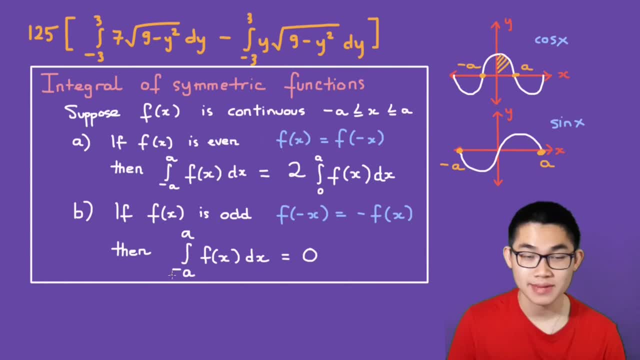 show that this formula is true, then the integral from negative a to a f of x, dx is equal to 0. so, for example, sine of x is an odd function. if this is negative a, this is a, then we know that. let's say, if we have to check the integration of the integral from the negative a to a, we know that. 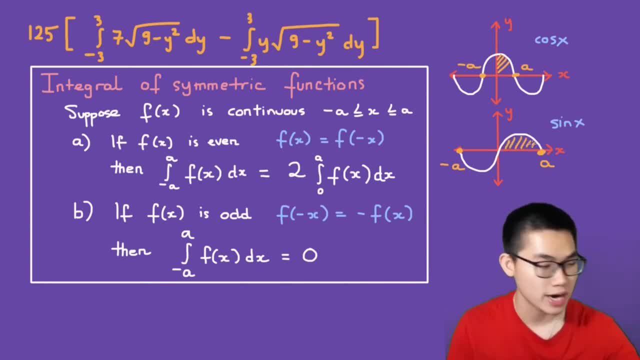 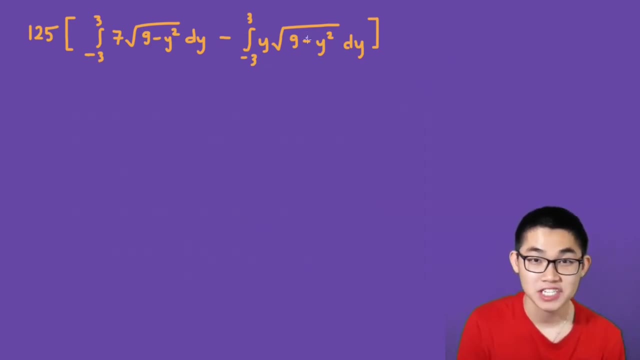 this area, let's say the area of that is 2, right well over here. the area here is negative 2.. so if you compute the integral from negative a to a, it's going to be 0. these two areas cancel out. if you look at this function, this is an odd function. it takes a little bit of practice. 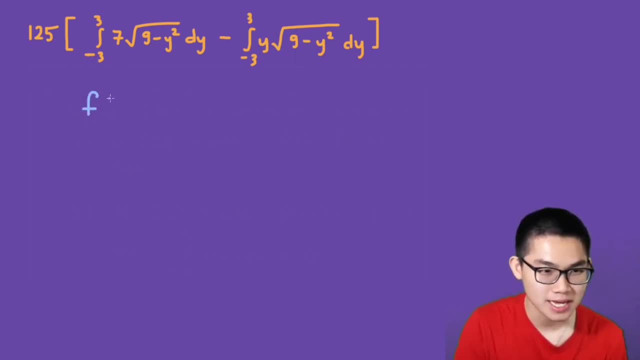 but let's prove that this is an odd function. so the formula is f of negative y, because it's, in terms of y, is equal to negative f of y. so here, f of y is this function, which is y times the square root of 9 minus y square. what is f of negative y? well, f of negative y is going to be what? well you. 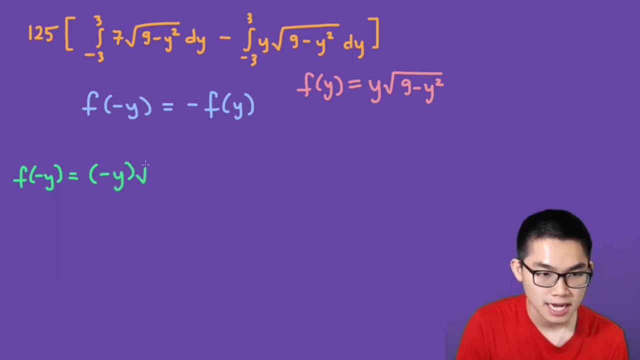 just replace the y with a negative y, like that times the square root of 9 minus negative y squared. so this is going to be negative y times 9 minus y square. how about negative f of y for this one? you just put a negative sign in front.